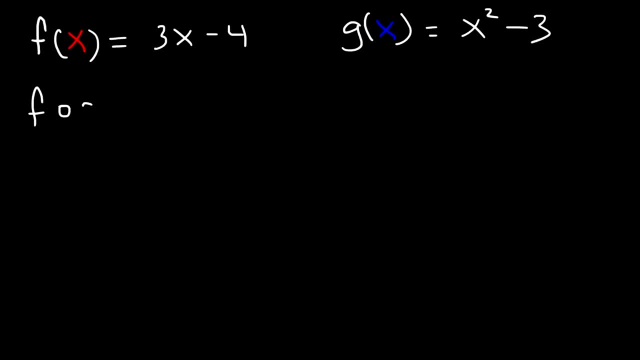 What is f of g? Notice that this is different from f times g. If you see a closed circle, it's multiplication. It's 3x minus 4 times x, squared minus 3.. But if you see like an open circle, what it means is it's a composite function. One function is inside of another. g is inside of f. 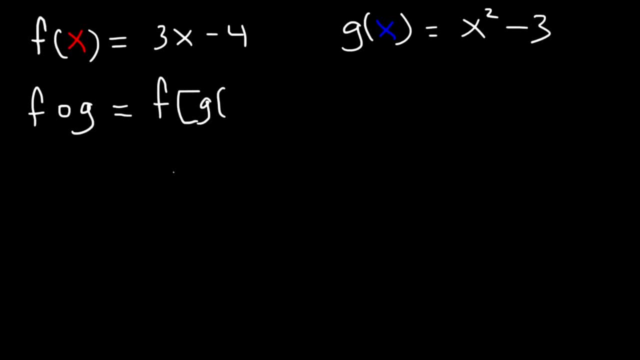 So this is equivalent to f of g of x. So how can we find f of g of x? Well, let's replace g. g is x squared minus 3.. And notice that x squared minus 3 is inside of f. So we're going to have to replace x with x squared minus 3.. 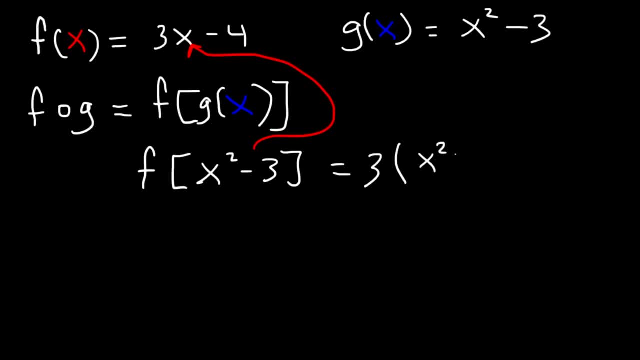 So this is going to be 3 times x squared minus 3 minus 4.. So now let's distribute the 3. So that's 3x squared minus 9 minus 4, which is 3x squared minus 13.. 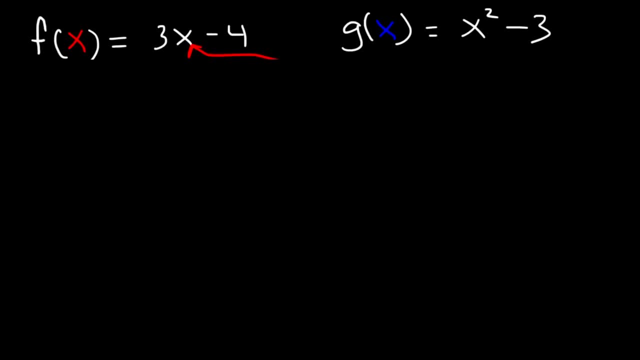 Now what about g of f? How can we find the value of g of f? So this time f is inside of g, So you can write it like this: That's an equivalent expression. Let's replace f of x with 3x minus 4.. 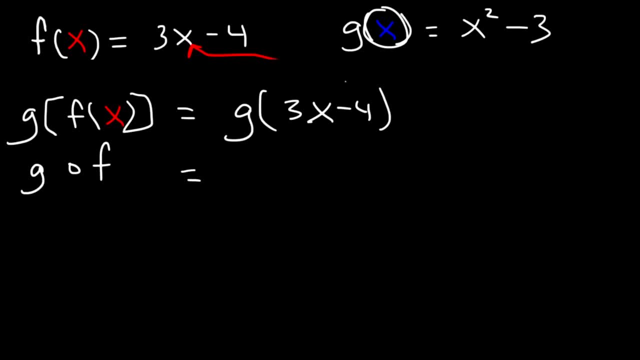 And now let's replace x with 3x minus 4.. So we're going to take this and plug it into here. So instead of x squared minus 3, it's 3x minus 4 squared minus 4.. 3x minus 4 squared is 3x minus 4 times 3x minus 4.. 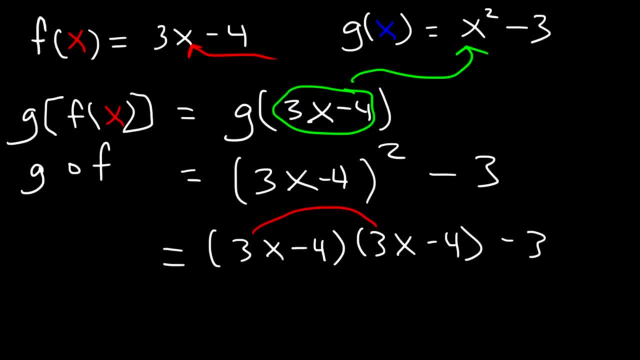 So if we FOIL it 3x times 3x, that's going to be 9x squared, And then 3x times negative 4, that's negative 12x. Negative 4 times 3x is also negative 12x. 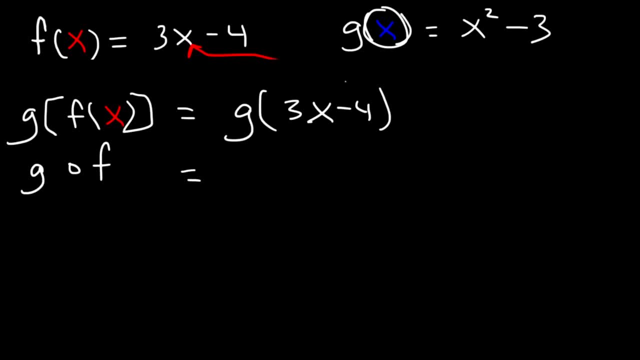 And now let's replace x with 3x minus 4.. So we're going to take this and plug it into here. So instead of x squared minus 3, it's 3x minus 4 squared minus 4.. 3x minus 4 squared is 3x minus 4 times 3x minus 4.. 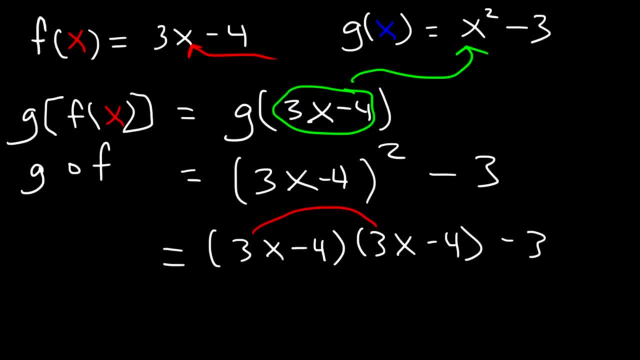 So if we FOIL it 3x times 3x, that's going to be 9x squared, And then 3x times negative 4, that's negative 12x. Negative 4 times 3x is also negative 12x. 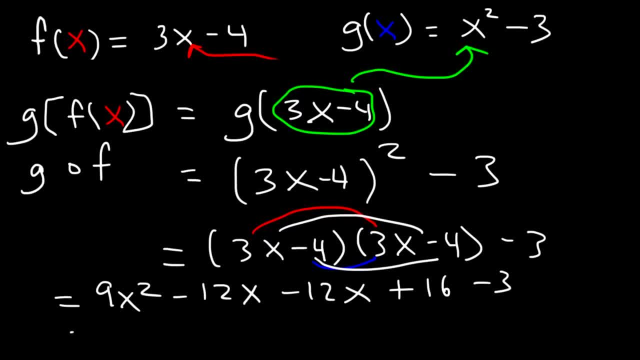 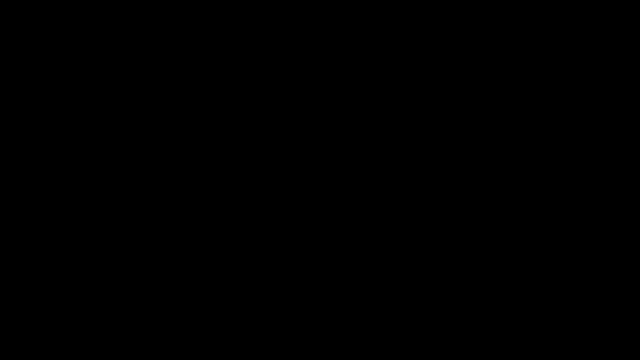 And then negative 4 times negative, 4 is 16.. Negative: 12 minus 12 is negative 4.. 16 minus 3 is 13.. So this is the value of g of f of x. Now let's say that f of x, let's say it's 5x plus 2.. 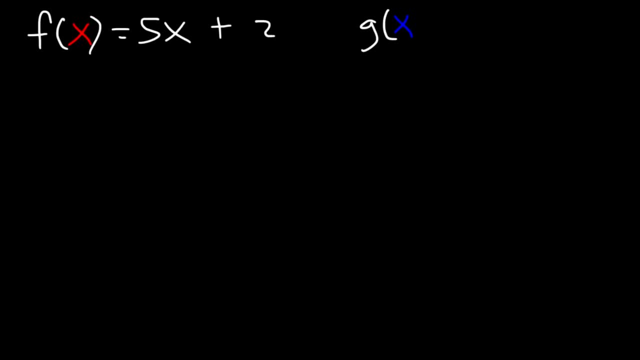 And now let's say that g of x is equal to x cubed minus 4.. Evaluate this function f of g of 2.. How can we do so? So first let's find the value of g of 2.. So let's replace x with 2.. 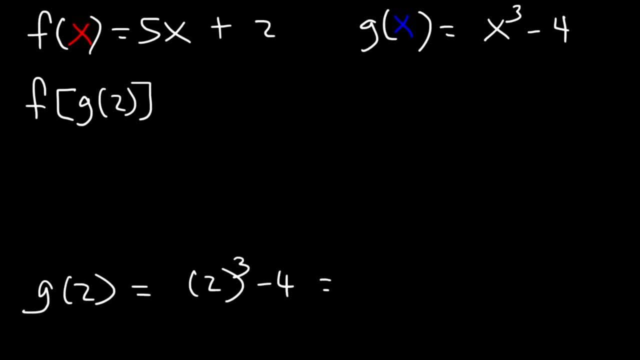 This is going to be 2 raised to the third power minus 4.. 2 times, 2 times 2, 3 times is 8.. 8 minus 4 is 4.. So g of 2.. So f of g of 2 is equivalent to f of 4.. 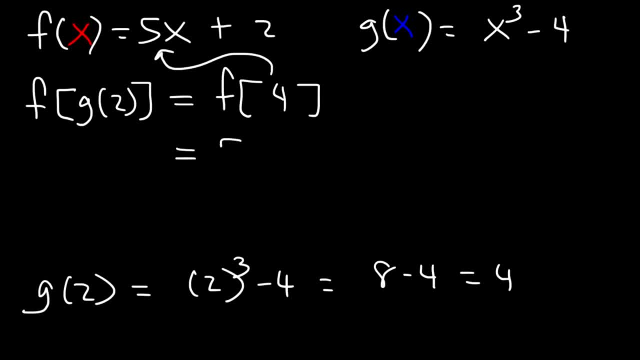 And now we can take 4 and plug it into that equation, So it's 5 times 4 plus 2.. 5 times 4 is 20.. 20 plus 2 is 22.. So that's how you can find the value of f, of g, of 2.. 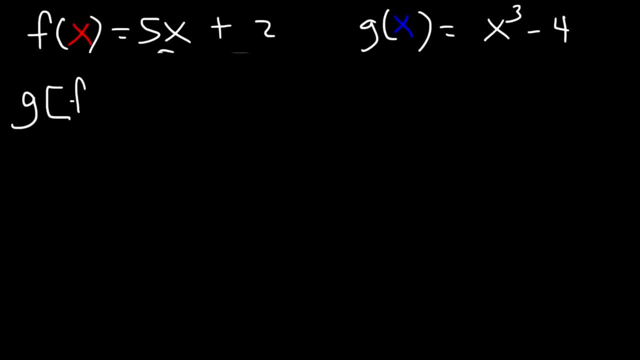 So try this one: Evaluate g Of f, let's say negative 1.. So first evaluate f of negative 1. That's 5 times negative, 1 plus 2. So make sure you're using this equation: That's negative 5 plus 2, which is negative 3.. 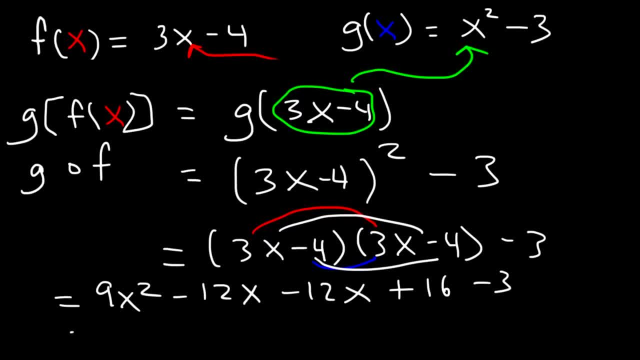 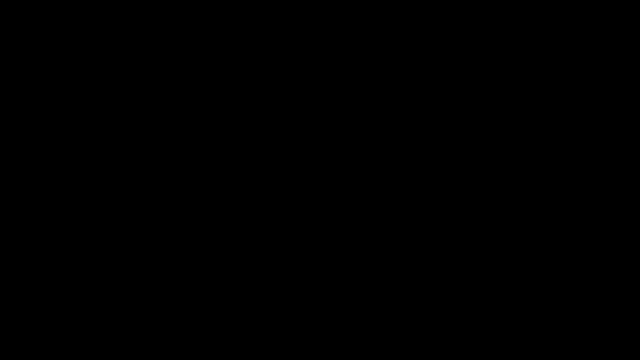 And then negative 4 times negative, 4 is 16.. Negative: 12 minus 12 is negative 4.. 16 minus 3 is 13.. So this is the value of g of f of x. Now let's say that f of x, let's say it's 5x plus 2.. 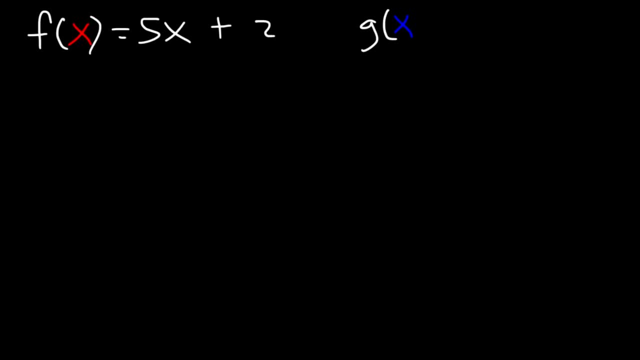 And now let's say that g of x is equal to x cubed minus 4.. Evaluate this function f of g of 2.. How can we do so? So first let's find the value of g of 2.. So let's replace x with 2.. 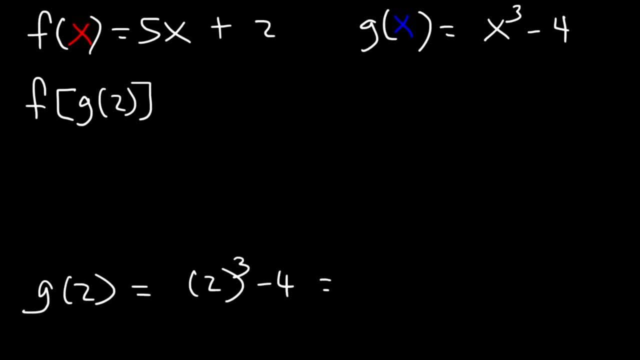 This is going to be 2 raised to the third power minus 4.. 2 times, 2 times 2, 3 times is 8.. 8 minus 4 is 4.. So g of 2.. So f of g of 2 is equivalent to f of 4.. 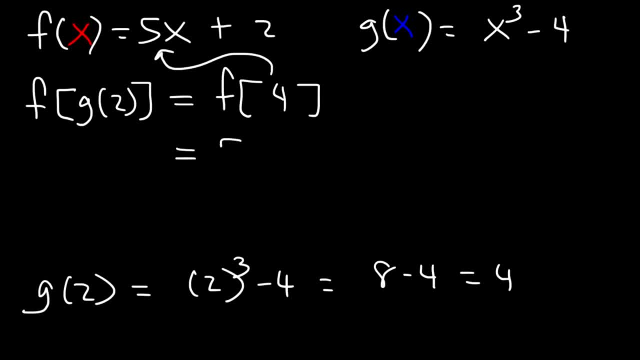 And now we can take 4 and plug it into that equation, So it's 5 times 4 plus 2.. 5 times 4 is 20.. 20 plus 2 is 22.. So that's how you can find the value of f, of g, of 2.. 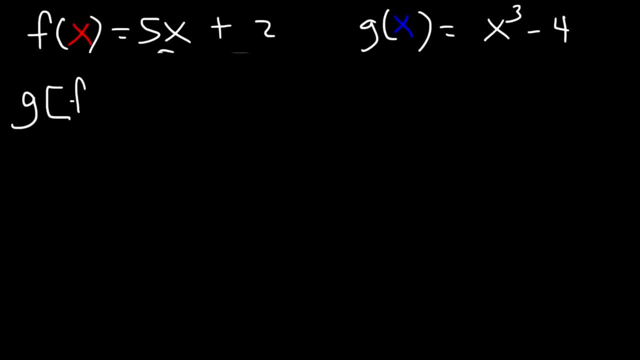 So try this one: Evaluate g Of f, let's say negative 1.. So first evaluate f of negative 1. That's 5 times negative, 1 plus 2. So make sure you're using this equation: That's negative 5 plus 2, which is negative 3.. 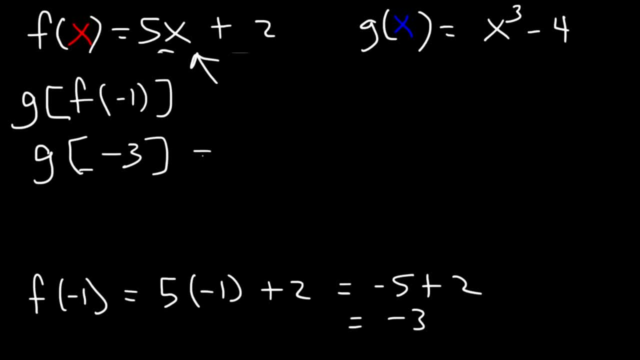 So f of negative 1, we can replace it with negative 3.. So now we're looking for g of negative 3, which we can plug it into here. So it's negative 3 to the third power minus 4, which is negative 27 minus 4.. 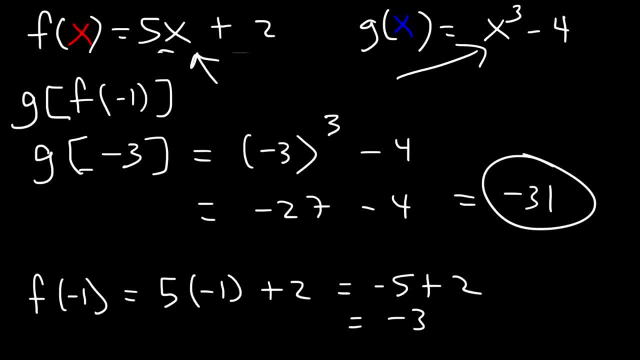 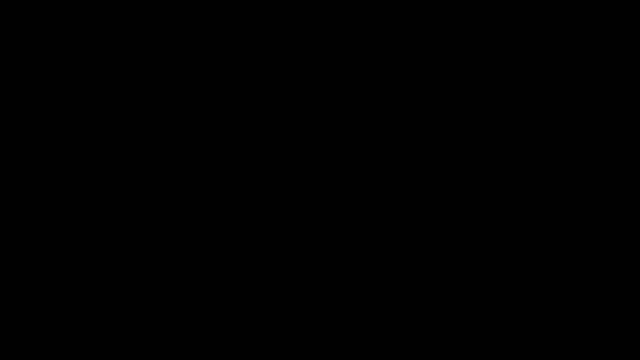 And so the final answer is negative 31.. So that's how you can evaluate composite functions. Thank you.